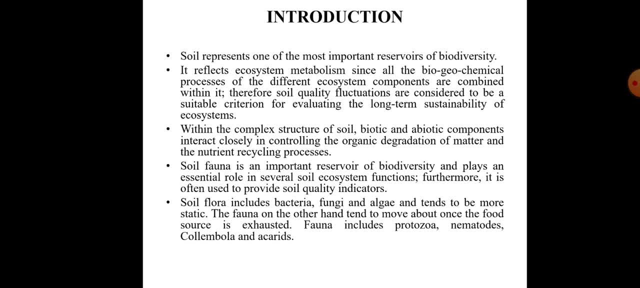 Ok, so firstly, their introduction. So soil represents one of the most important reservoirs of biodiversity. It reflects ecosystem metabolism, since all the biogeochemical processes of the different ecosystem components are combined within it. Therefore, soil quality fluctuations are considered to be a suitable criterion for evaluation. 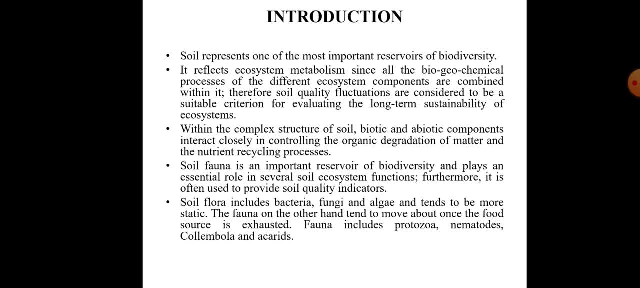 As well as evaluating the long term sustainability of eco-system. Within the complex structure of soil, biotic and abiotic components interact closely in controlling the organic degradation of matter and the nutrient recycling processes. Soil fauna is an important reservoir of biodiversity and plays an essential role and important role in several soil commandments, such as soil biocomposition and marine civilizations. 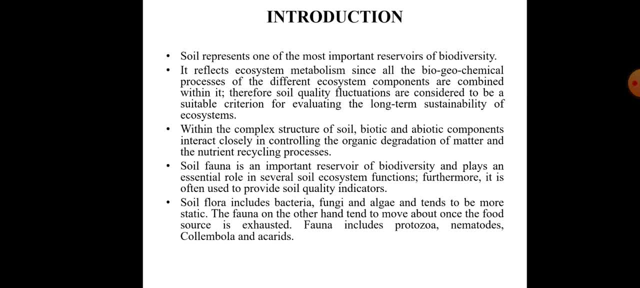 And in some areas soil or Af demás, also needs numbering and spatialçeak role for a development including biodiversity conservation and organic celleification. Soil bitterness is common and an essential resource in stacked hallucinogens and famine. Soil vertes important natural liksom하세요ly. 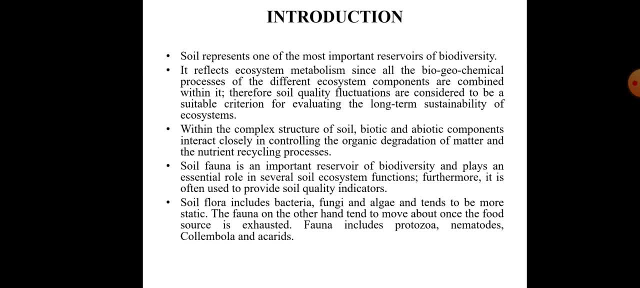 soil ecosystem functions. furthermore, it is often used to provide soil quality indicators. then soil flora includes bacteria, fungi and algae, and tends to be more static. the fauna, on the other hand, tends to move about once the food source is exhausted. then fauna includes predators, protozoa, nematodes, then columbola, then acarids. ok, so these are the some examples. 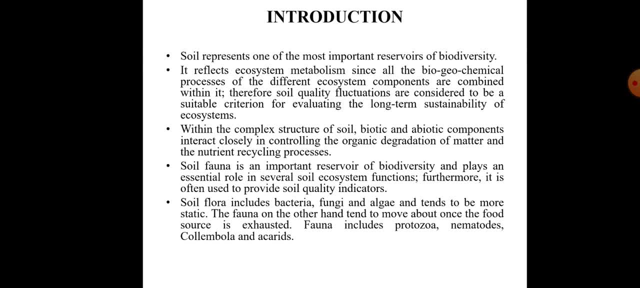 of soil flora. ok, so in the soil or in the ecosystem there are chemical processes and cycles. ok, so these all are dependent to each other. whether it is soil or air or water, there are chemical cycles. in the soil or in the ecosystem, biochemicals or biogeochemical processes are all dependent to each other, right, so that's? 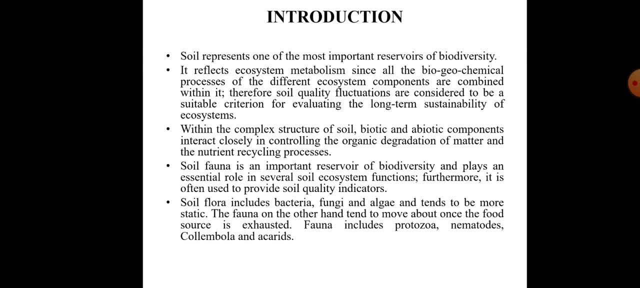 why soil also represents one of the most important reservoirs of biodiversity. right so in the ecosystem there will be biotic components or abiotic. that means living or non-living components. some structure or maintenance of the soil, or even the fertility of the soil are all effected on the soil. right then organic degradation of matter and the nutrient recycling. 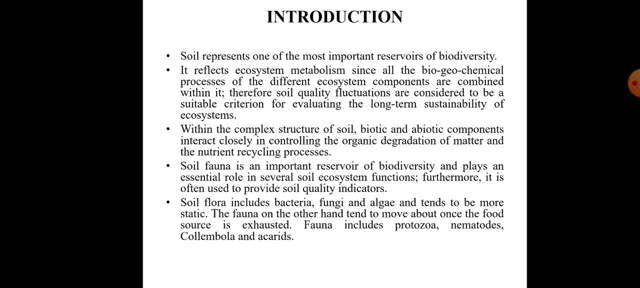 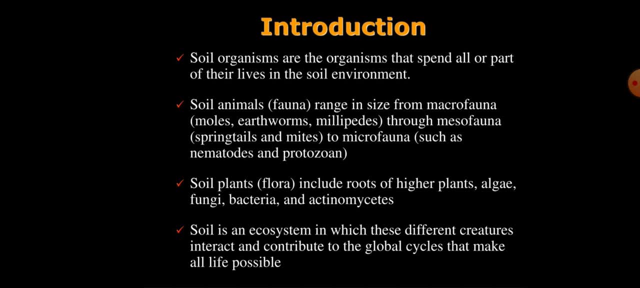 processes. these all are interact with biotic or abiotic factors. okay then, soil organisms are the organisms, Sok, that spend all or part of their lives in the soil environment. soil animals, that means fauna, range in size from macrofauna, that is, moles, earthworms, millipedes, okay, through mesofauna. 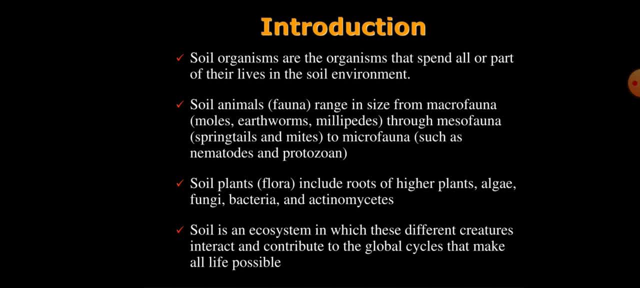 their example springtails and mites. okay, to microfauna such as nematodes and protozoans. right, so then soil plants, that is flora, include roots of higher plants, then algae, fungi, then bacteria and actinomycetes. okay, so these are the soil flora and soil fauna. 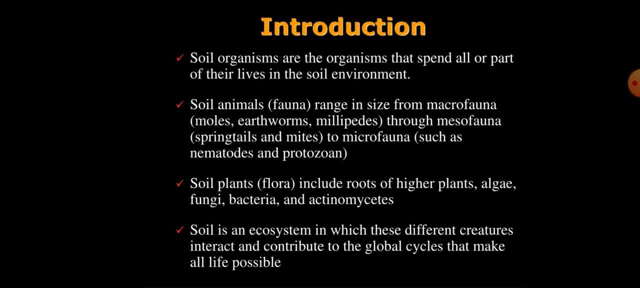 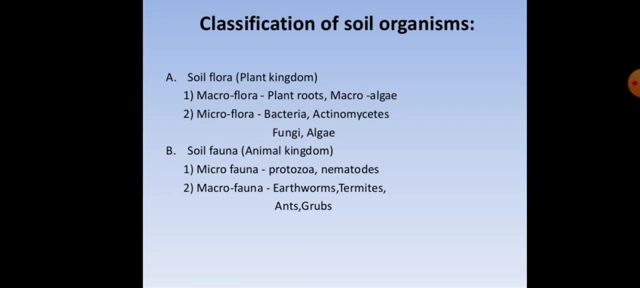 and their example. so soil is an ecosystem in which these different creatures interact and contribute to the global cycles that make all life possible. okay, so this is the introduction of soil Torah of soil flora and soil fauna. ok, so next one is classification of soil organisms. firstly, soil flora in plant kingdoms: first one, macro fauna, and second one is micro fauna. so firstly, 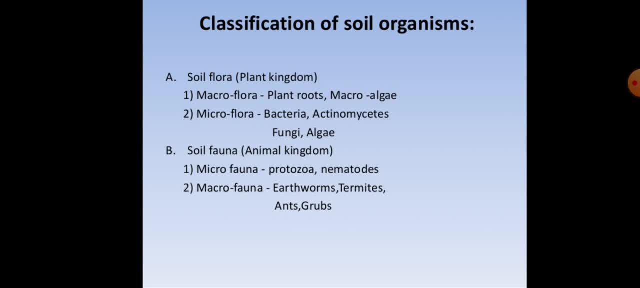 macro fauna. flora is plant roots and macro is algae. ok, then micro flora- bacteria, actinomycetes, fungi and algae. ok, these are the examples of macro and micro flora. ok, so then next classification is soil fauna- animal kingdom. ok, so these are also two types: micro fauna and macro fauna. 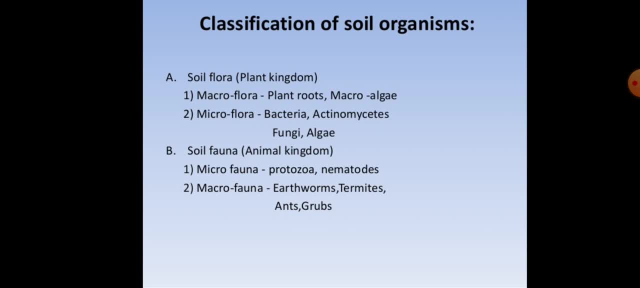 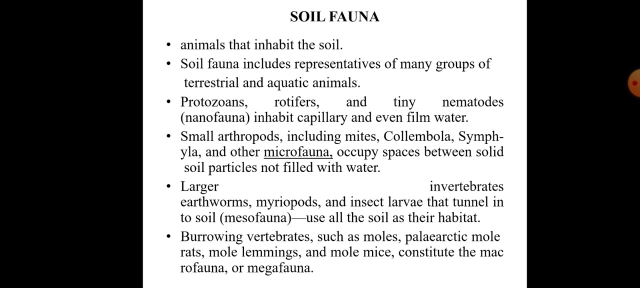 micro fauna. micro fauna examples protozoans and nematodes, and then macro fauna, earthworm and termites, ants, grubs. these are the examples of soil fauna. ok, then, firstly, soil fauna, animals, that of the inhabits the soil. so soil fauna includes representative of many. 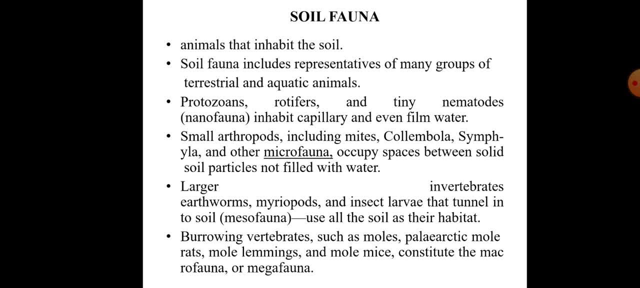 groups of terrestrial and aquatic animal. ok, so protozoans, rotifers and tiny nematodes, that is, nanofauna, inhabit capillary and even film water. ok, small orthopods, porous then, including mites, colembolaishos and ptites, etc. etc. of Eucalyptuses, yep, other species. 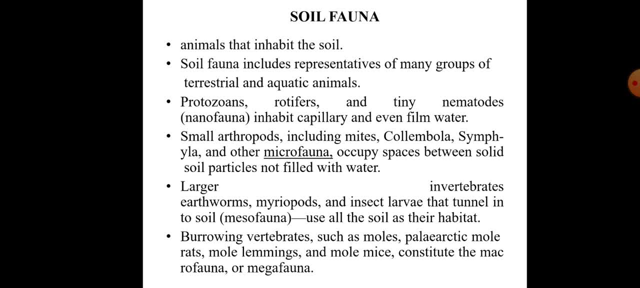 that you see sketchlist and picture. clarification of soil fauna. Isaach, vemos ones called nanofauna, Then Symphoila and other microfauna occupy spaces between solid soil practice particles not filled with water. ok, Then larger invertebrates, that is, earthworms, then myriopods and insect larvae that tunnel. 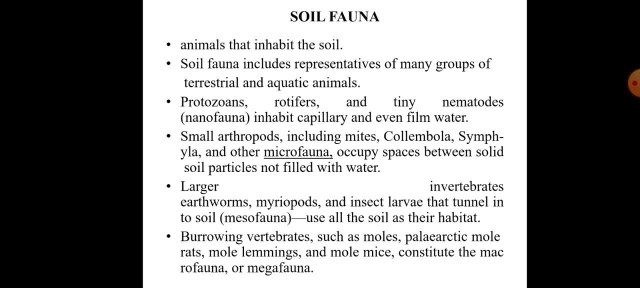 in to soil. that is mesofauna use all the soil as their habitat. So the larger invertebrates, earthworms, myriopods and insect larvae that tunnel in to soil. that is mesofauna use all the soil as their habitat. ok. 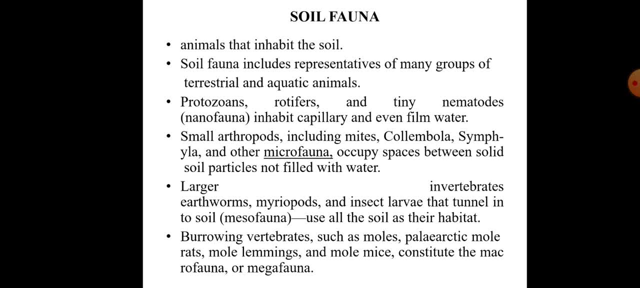 So burrow invertebrates such as moles, then palaeeretic moles, rat, then mole lemoning and mole mice constitute the macrofauna and megafauna. ok, So these are the soil fauna, ok, Animals that inhabit The soil. 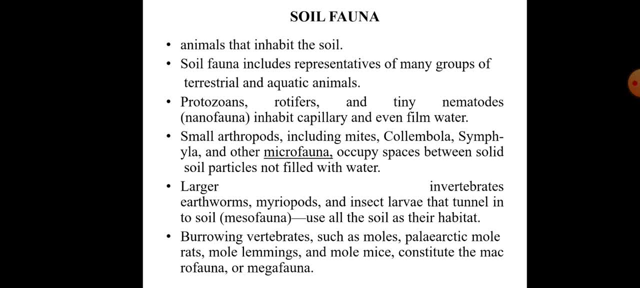 The animals that are present in the soil, like the protozoans, rotifers and tiny nematodes- ok. Then the small earthworms, including mites, columbola, then Symphoila and other microfauna. these all are the existing fauna, ok. 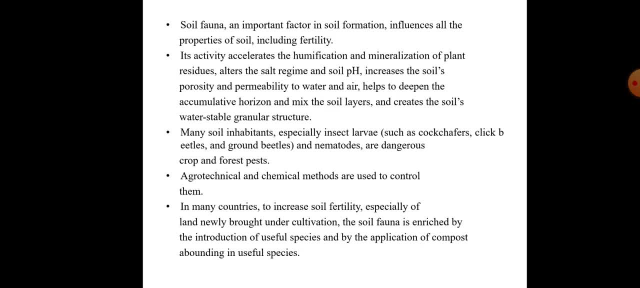 These are the examples of soil fauna. ok, So soil fauna, an important factor in soil formation, influences all the properties of soil, including fertility right. Its activity accelerate the humification and mineralization of plant residues, alter the salt regime and soil pH, increases the soil's porosity and permeability to water and air. 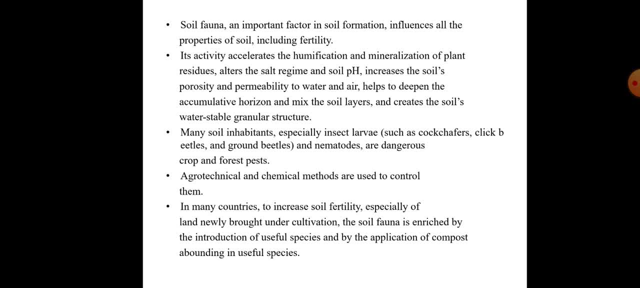 helps to defend the accumulative highlighting and strips skin body and helps to reduce semen decompositionェ. об foremost of the soil schema cah, because a change and Tempest is felt in soil and mix the soil layers and creates the soils, water, stable, granular structure. 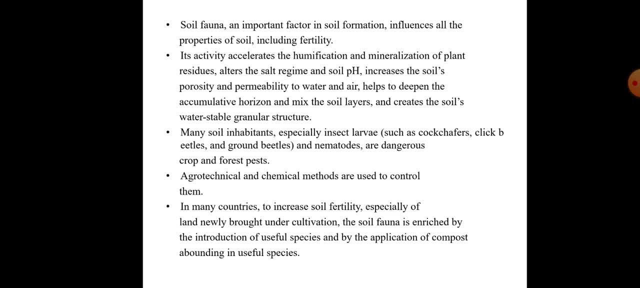 okay many soil inhabitants, especially insects, larvae such as cock chaffers, then click be, click beetle and ground beetles okay. and nematodes are dangerous crop and forest paste, then agrochemicals and an agro technical and chemical methods are used to control them in many countries to increase soil fertility. 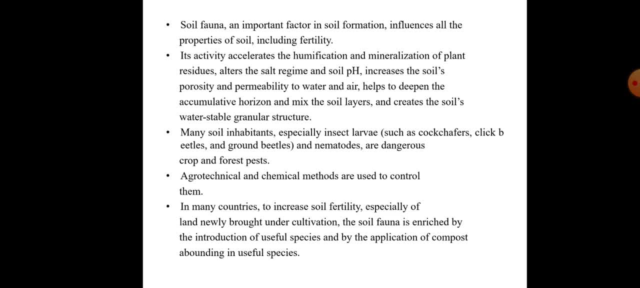 especially of land newly brought under cultivation. the soil fauna: it's enriched by the introduction of useful species and by the application of compost abounding in useful spaces. okay, so these are the soil fauna that is important role. okay, so these are the soil fauna that is important role. 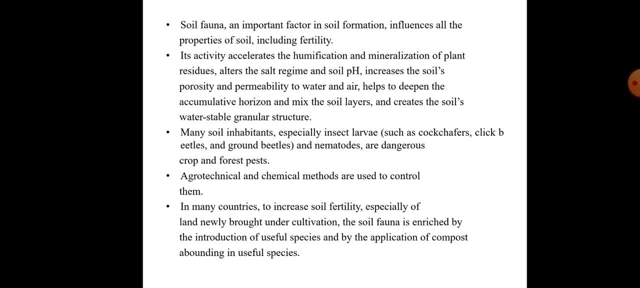 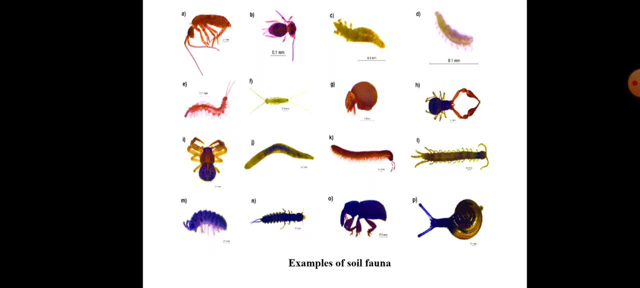 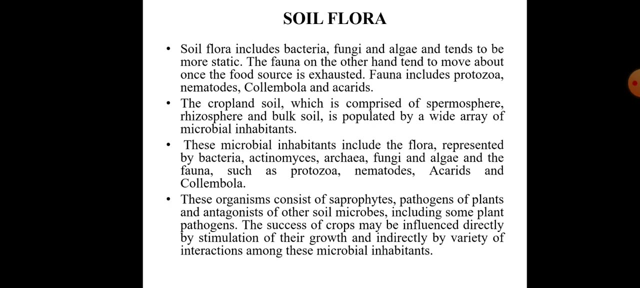 okay, so these are the soil fauna that is important role playing in the soil fertility properties of soil. ok then, soil formation. right, these are the some examples of soil fauna. ok, then, next one is soil flora. soil flora includes bacteria, fungi and algae, and tends to be more static. the fauna, on the other hand, tends to move. 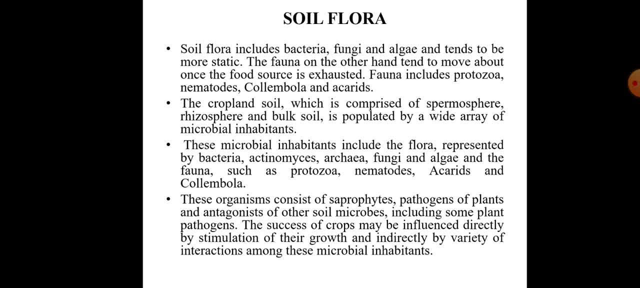 about once the food source is exhausted. fauna include protozoa, nematodes, then columbola and acarides. ok, these are the some examples of soil flora. the cropland soil, which is comprised of spermosphere, rhizosphere and bulk soil, is populated by a wide array of microbial. 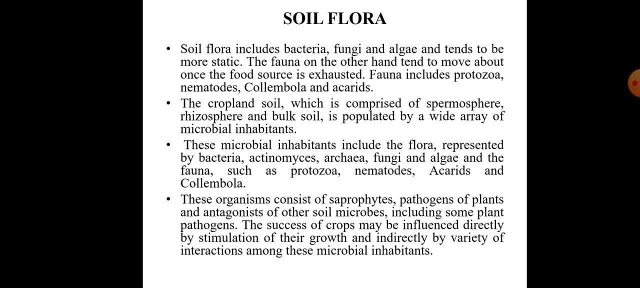 inhabitants. these microbial inhabitants include the flora, represented by bacteria, actinomycetes, then archaea, then fungi and algae, and the fauna, such as protozoa, nematodes, acaride and columbola ok. these organisms consist of saprophytes, pathogens of plants and antagonists of other. soil microbes, including some pomegranates. ok, so for cleaning this soil, which are soil rock, very important. so we are going to clean soil with so little. then, over the next few days, we are going to clean it, and so we are going to clean the soil with a spray of it. can you believe this is a white colour? okay, so we are going to wipe the soil with a wet or a dry brush. wet brush, or you can remove this, if you want to, and then leave it on the bed and you can see the visible surface of the soil, or you can see the residue of earthy 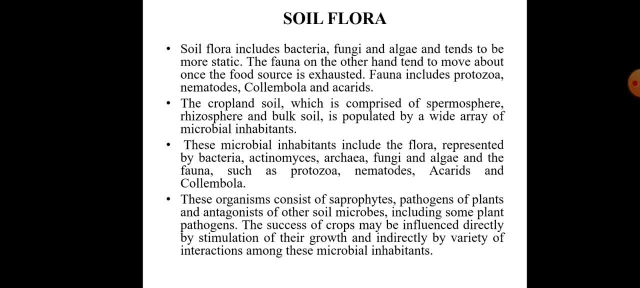 plant pathogens. the success of crops may be influenced directly by stimulation of their growth and indirectly by variety of interactions among these microbial inhabitants. okay, so soil flora is also important, playing important role in the soil fertility, as well as soil structure, as well as soil maintenance as well. okay then, soil fertility right and the some. 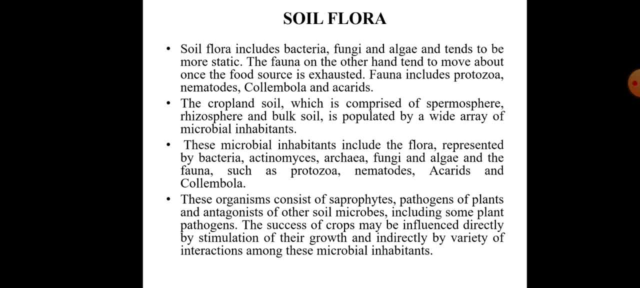 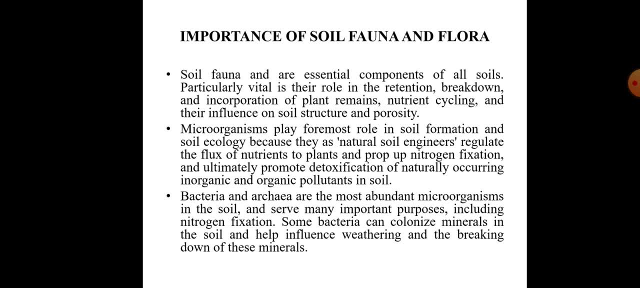 examples of soil flora, that is, the algae, fungi, bacteria. okay then, next one is importance of soil fauna and flora. so soil fauna and are essential component of all soils. particularly vital is their role in the retention, then breakdown and incorporation of plant, remains nutrient cycling and their influence on soil structure and porosity. okay, japan, soil fauna. 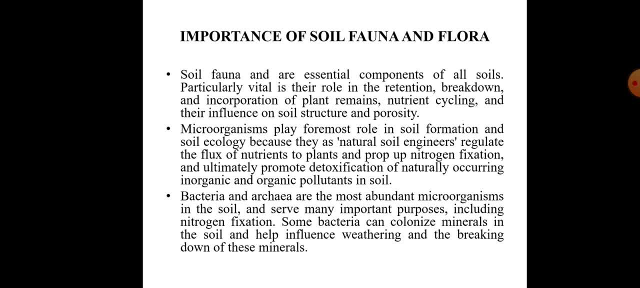 flora as well as soil flora. so soil flora is important role in the soil fertility and they are very, they are playing very important role in the and their retention, then breakdown and incorporation of plant remains and their nutrient cycling and their influence influence on soil structure, as well as soil легibility and porosity as well. right then, microorganisms play foremost. 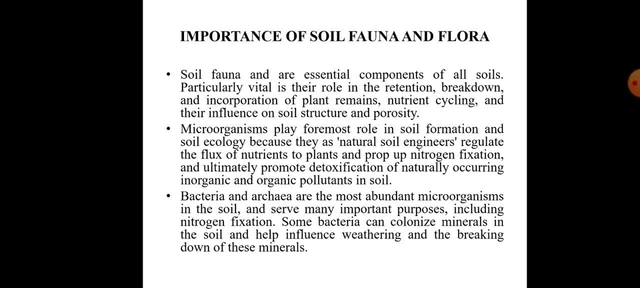 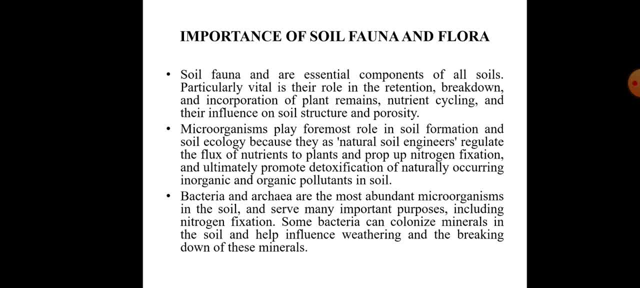 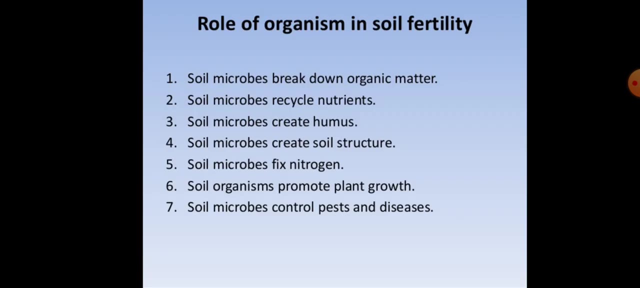 then next one is bacteria and archaea are the most abundant microorganisms in the soil and serves many important purposes, including nitrogen fixation. some bacteria can colonize minerals in the soil and help influence weathering and the breaking down the of these minerals. okay, so these are the some importance of soil fauna and the flora. okay, then next one: role of organisms.